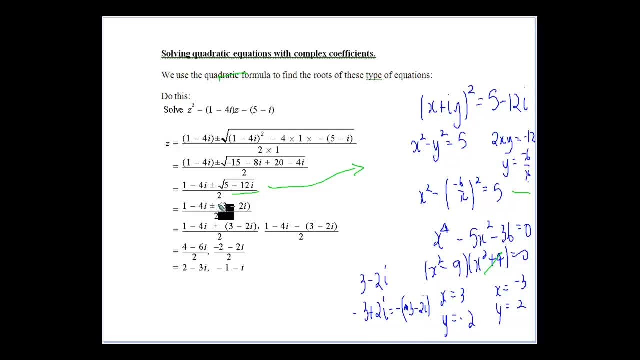 minus outside of 3 minus 2i. this is why we write it like that: minus plus, or minus 3 minus 2i, because it gives me those two solutions which were the solutions given to us there. so split it up, because we're going to have two separate solutions here. so 1 minus 4i plus 3 minus, so i can collect our. 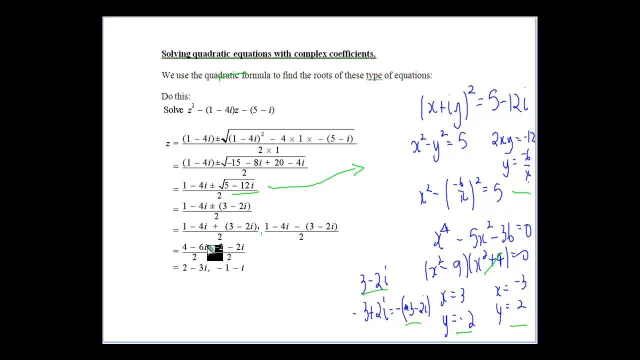 terms our real parts and collect our imaginary parts: 4 minus 6i on 2. 4 divider by 2 to give you 2 minus 6, divided by 2, to give you minus 3, and then we have the 1 minus 3 gives us minus 2, minus 4. minus minus 2 gives us a minus 2i. so and then, 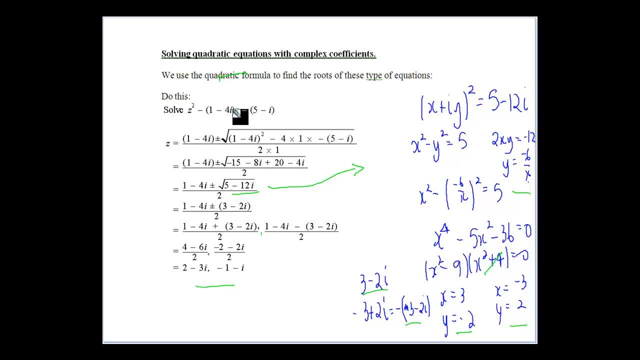 divide both sides by 2, there's our two solutions to that quadratic. now that's not that's. that's a lot of work involved, because you've got to do a separate process of that to get the solutions to that square root of the quadratic. so that's where, with that, that part's definitely going to come in. 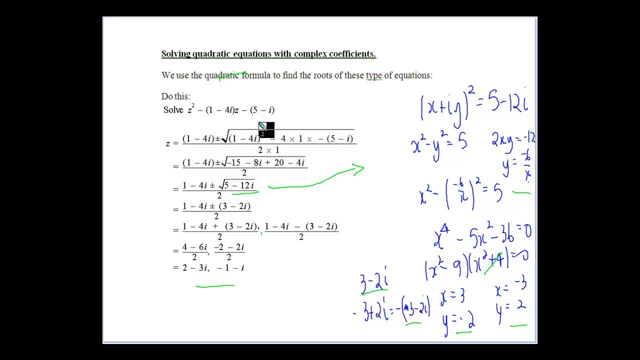 to solve equations like that. what we said before about appearing as complex conjugates not occurring in this game, because they are root, because they are coefficients, are complex, that rule only work. that rule doesn't work here, any works when we've got roots of our, of our, the coefficients of our equations, or 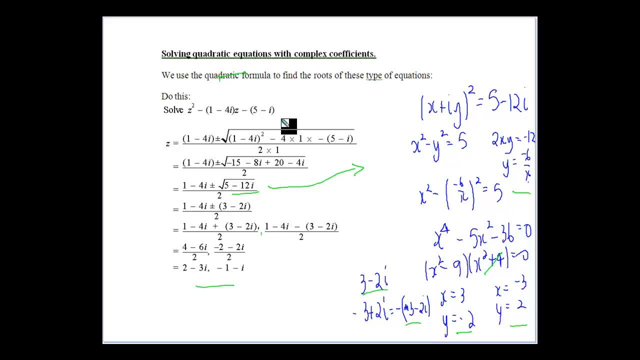 polynomials, whatever we want to look at being. you know, if you're going to be able to do this, you're going to have to do this. you're going to have to do this, you're going to have to do this. real numbers, okay, so they're not going to occur in complex, complex conjugate. 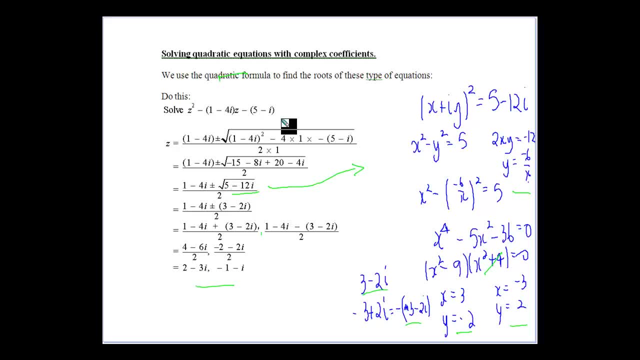 pairs makes life a little bit harder, but we can't do much about that. so there's that process there. we need to be able to solve quadratic equations with complex coefficients.